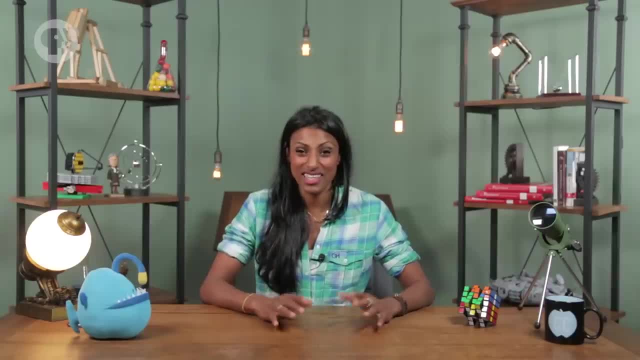 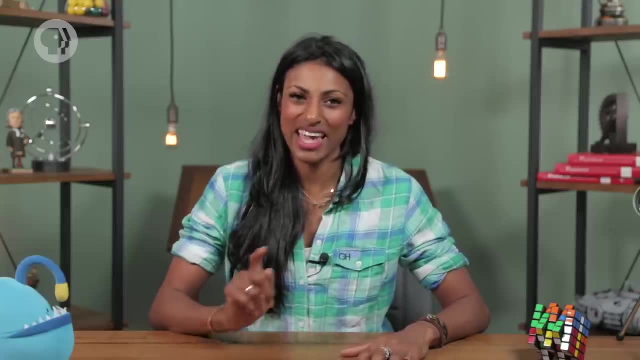 It's called momentum, and it's one of those things that's easier to see in real life than to describe. Momentum is often described as an object's tendency to remain in motion, but technically it's an object's mass times velocity, So a big bag full of leaves rolling down a hill. 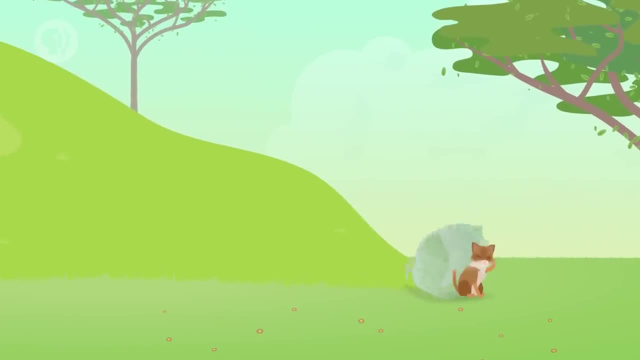 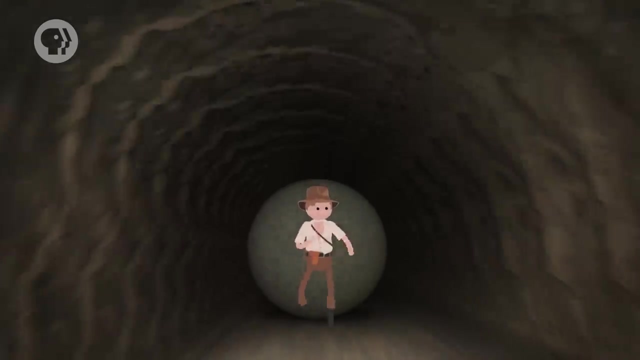 It might be going fast but it doesn't have much mass, so it doesn't have a lot of momentum And it wouldn't be too hard to stop. But the boulder chasing Indiana Jones, That had a lot of mass And therefore lots of momentum. So it would have been much harder to stop, And momentum is one factor that affects collisions between objects. After all, if a huge boulder crashes into another huge boulder, that's going to be a very different sort of crash than if a bag of leaves crashes into a boulder. 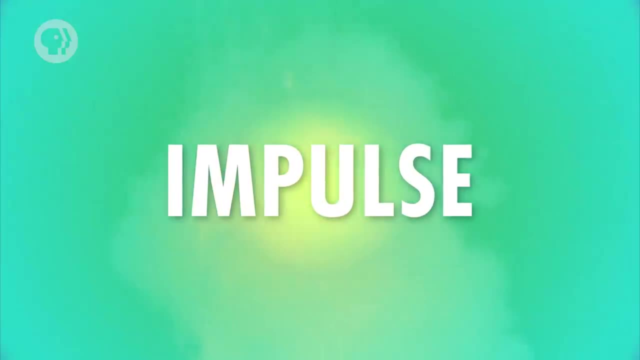 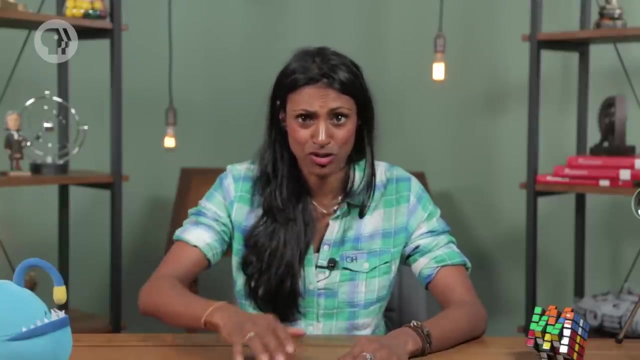 But the other quality of a collision that we often consider is known as impulse, which, at least in the context of physics, doesn't actually have anything to do with willpower Or why you throw your game controller when you get stuck on a level. 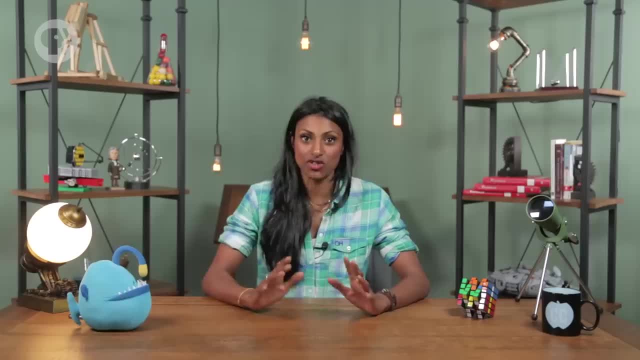 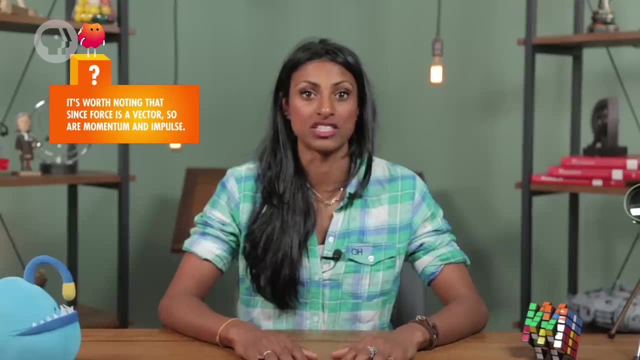 Instead impulse…. …usually represented by momentum. Impulse, represented by a j, is the integral of the net force on an object over time, In other words, it's change in momentum. Impulse turns out to be a particularly useful way to describe a crash because generally in collisions, forces change very quickly. 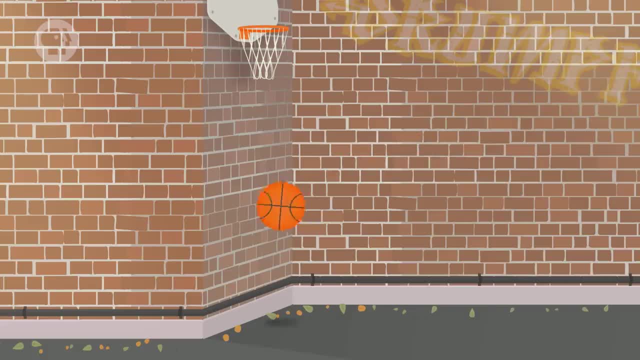 So if a ball smacks into a wall and over the course of half a second its force on the wall in newtons is equal to the time multiplied by 25, we'd say that its impulse was 3.1 newton-seconds. 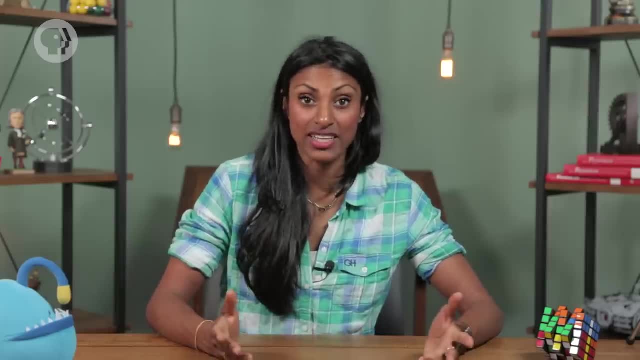 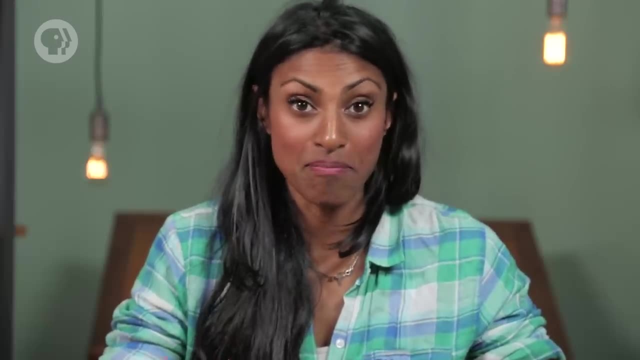 Now let's consider the different kinds of collisions that we can study. Generally, collisions can be described as either- And it's going to be important to figure out which kind you're dealing with, because the math works in very different ways. If elastic collisions sound bouncy, that's because they are. 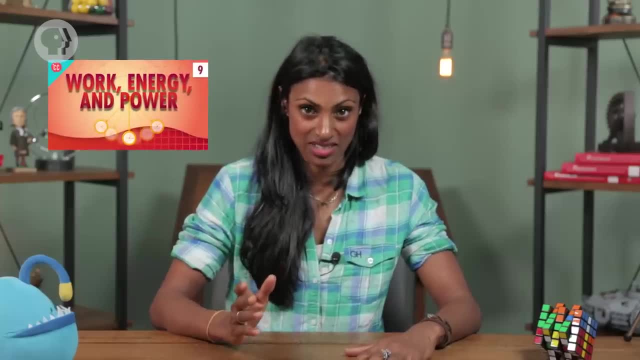 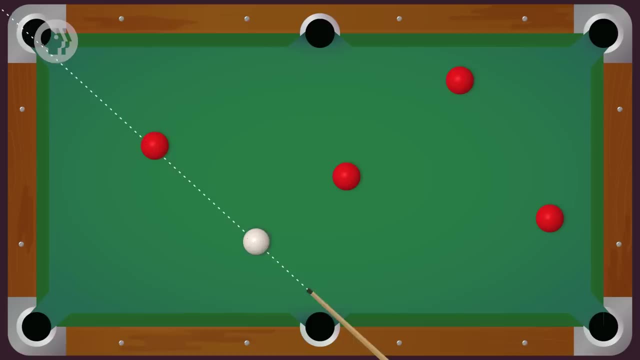 Like the conservative systems we talked about last time, in elastic collisions kinetic energy is neither created nor destroyed. For example, let's say you knock a white billiard ball into a second red one that's sitting on the table and they hit each other in just the right way. 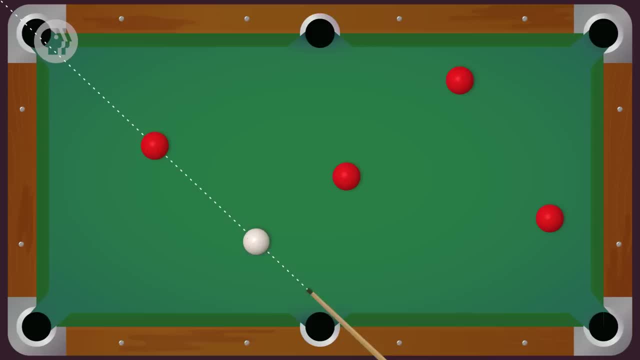 For this to be a true elastic collision, all of the kinetic energy from the white ball would have to be transferred to the red ball, Meaning that after they hit each other, the white ball would stay put and the red one would zoom away with all of the kinetic energy. 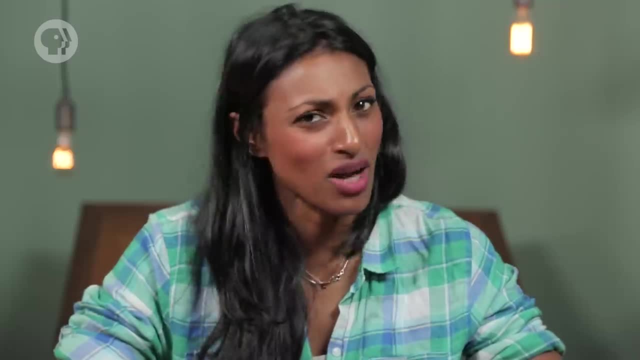 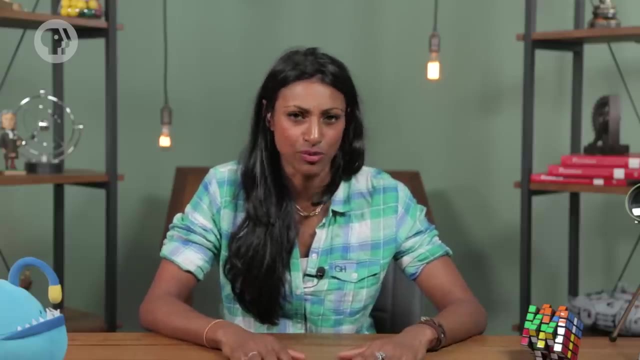 So the same speed, basically, that the white ball used to have. But you won't come across elastic collisions in real life, Because there's always going to be some energy that's lost somewhere in the collision, Generally lost as heat or sound. 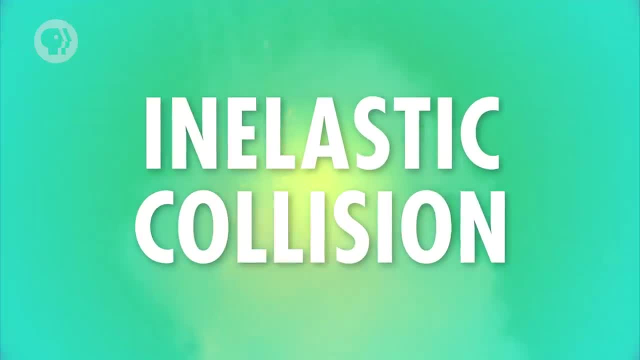 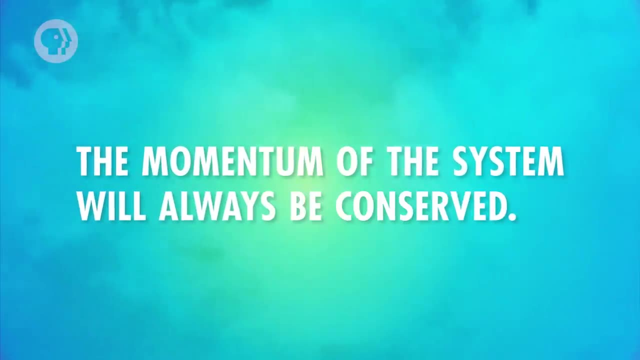 And when kinetic energy isn't conserved, that's an inelastic collision. There is one thing that's going to be true about every collision: Whether or not it's elastic, the momentum of the system will always be conserved. It might be transferred to another object. 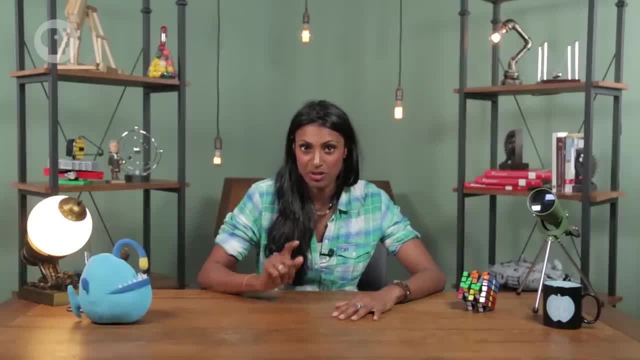 It might even be transferred to another planet. It might even be transferred to another R1.. It might even be transferred to another planet. It might even be transferred to another planet, transferred to more than one object, but the momentum is always going to go somewhere. 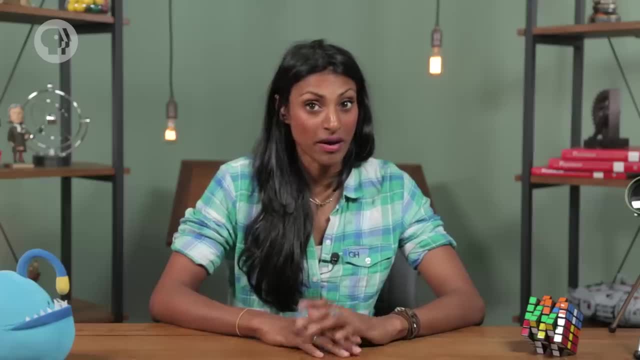 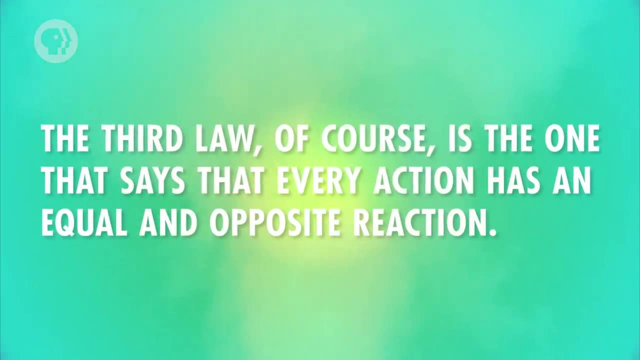 And we'll be able to use math to figure out where it went. Plus, we can use what we know about impulse and Newton's third law to prove it. The third law, of course, is the one that says that every action has an equal and opposite reaction. 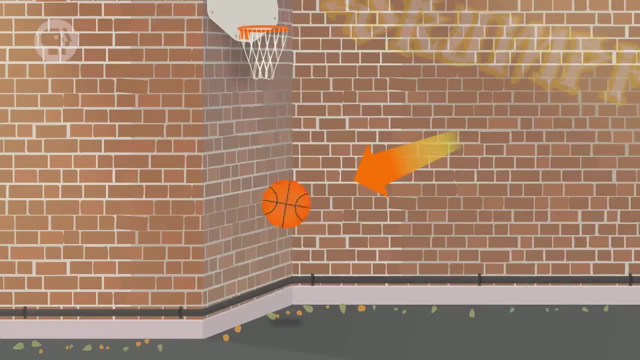 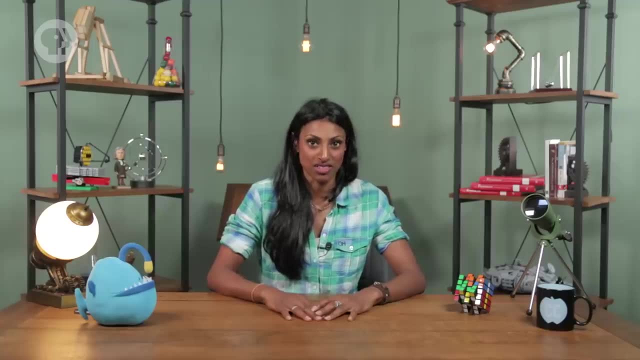 And that applies to collisions in the same sense that if a ball hits a wall, it'll exert a force on the wall and the wall will exert an equally strong force back on the ball. We can describe each of these forces as impulses, since we know that an impulse is just a change. 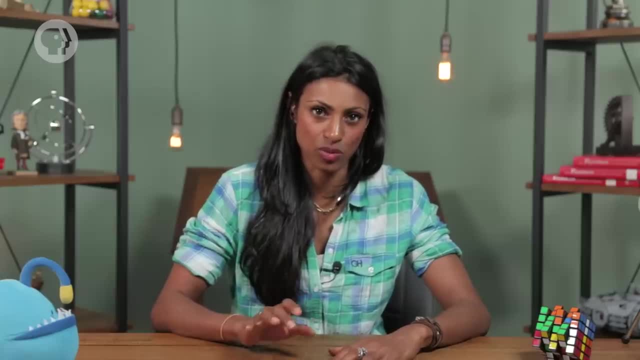 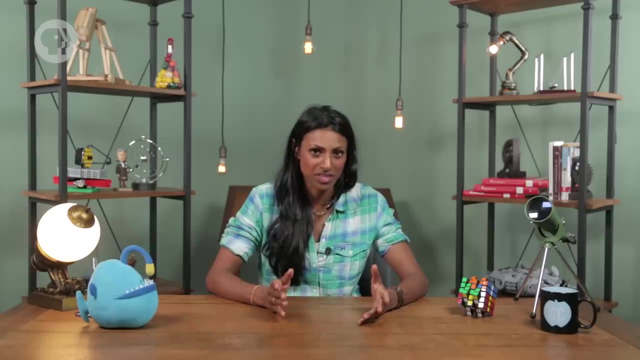 in an object's momentum. So the ball's momentum will be decreasing when it hits the wall. But because of Newton's third law we know that the wall's momentum is going to increase by an equal amount. The change in the wall's momentum might be impossible for us to see, because the wall 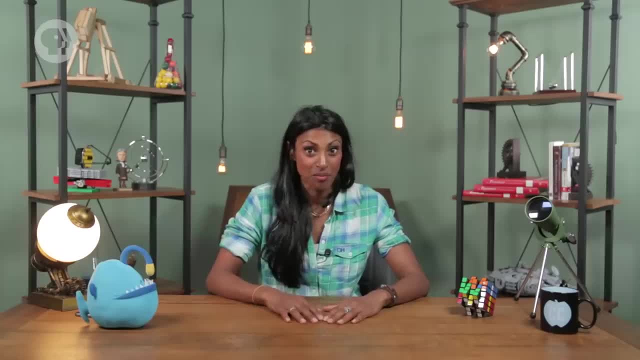 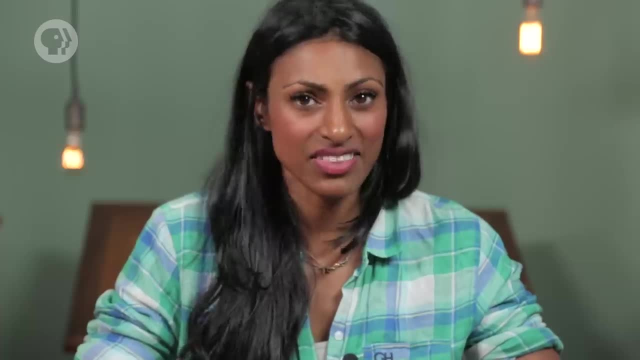 is connected to the ground and the Earth has lots of mass, But it's there, And that fact that momentum is always conserved turns out to be super helpful for describing collisions using math, Like in the case where you knocked the white billiard ball into the red one. 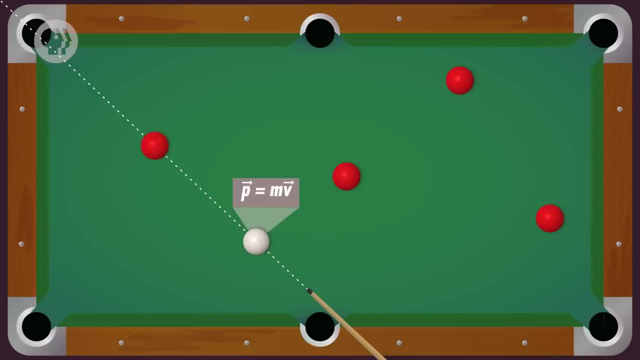 Since momentum is conserved and momentum is mass times velocity, the white ball's mass times velocity burns Before the collision. it has to be equal to the mass times velocity plus the red ball's mass times velocity after the collision, Which is why, assuming the balls have the same mass, if the white ball stops moving. 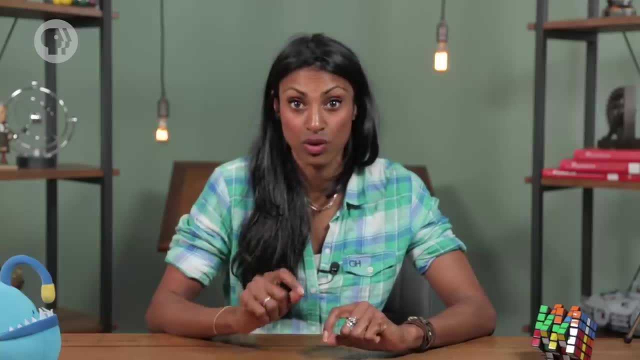 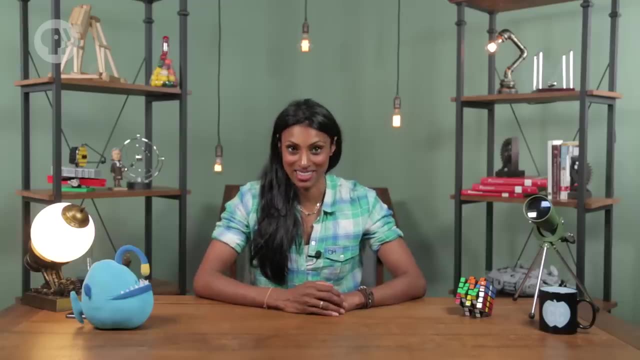 after the collision, then the red ball must move with the same velocity that the white ball had. So now we know about both elastic and inelastic collisions. But there's also such a thing as a perfectly inelastic collision, because… of course there is. 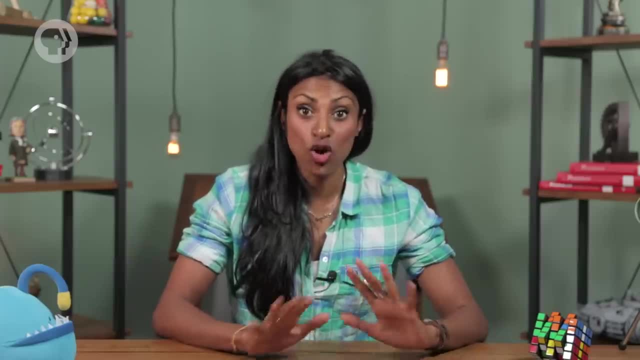 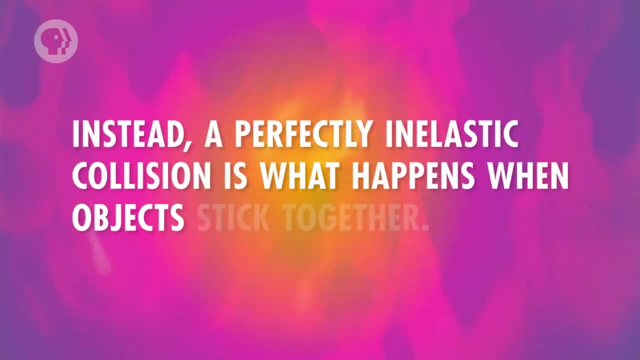 And it's easier for me to tell you first what it isn't. So it is not a collision where the objects lose order. Instead, a perfectly inelastic collision is what happens when objects stick together. These collisions lose as much kinetic energy as possible to other forms of energy, like 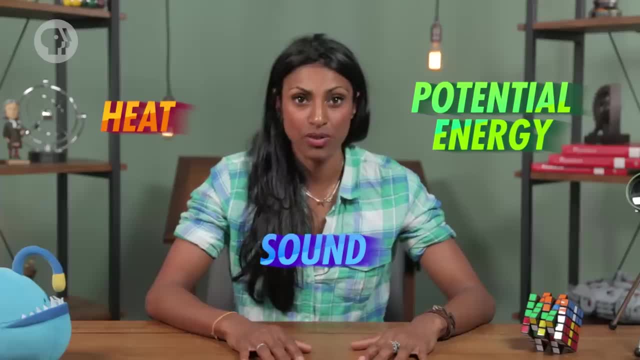 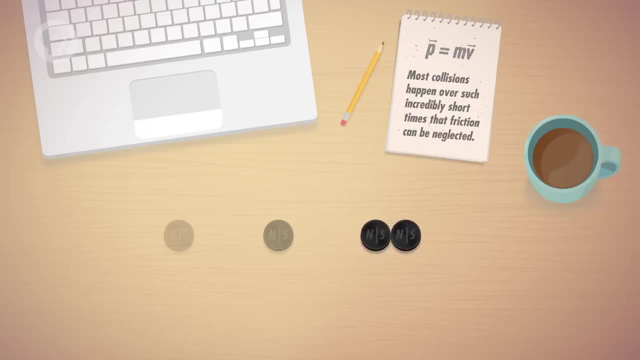 heat or sound or even potential energy, But still their momentum is conserved. An example would be if you pushed one magnet towards another at just the right angle for them to stick together on contact, and then they both started sliding together at half the speed of the magnet you pushed. 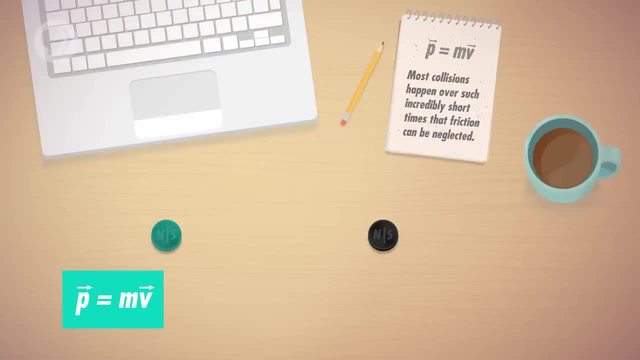 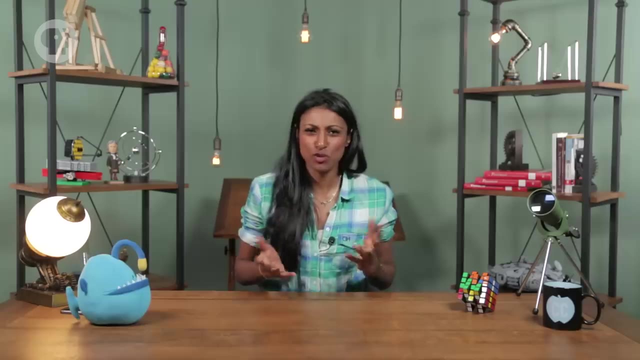 Before the collision, the momentum of one magnet was zero and the momentum of the one you pushed was its mass times velocity. Once the magnets collide, the mass is doubled and the velocity is cut in half. So the total momentum stays the same, but you lose some kinetic energy because there's 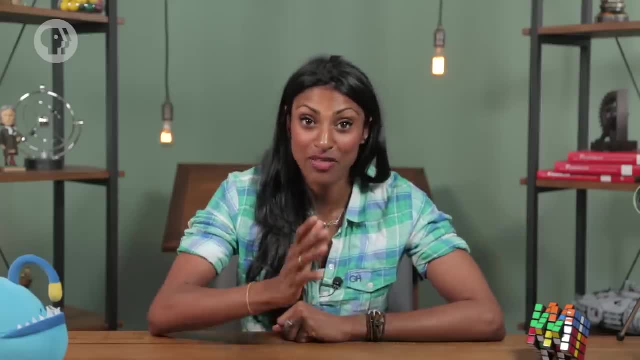 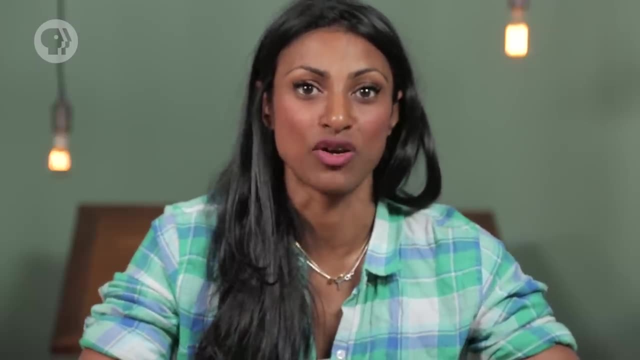 less speed involved. So that's the basics of how collisions work and how they relate to the momentum of motion in a straight line. But there's one more detail we have to explore in order to really understand how objects move, whether they're going to collide or not. 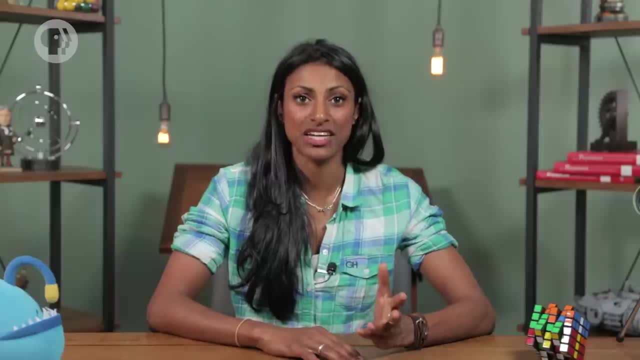 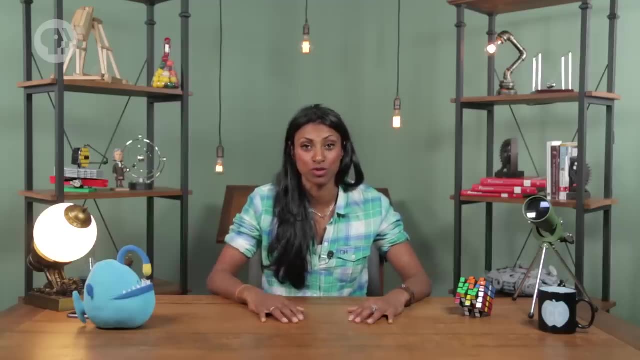 And that is center of mass. Until now we've been talking about objects as though they were little pinpoint particles, And that's worked for us. And that's worked fine for the most part, because the objects we've been talking about would act much like a small dot, would. 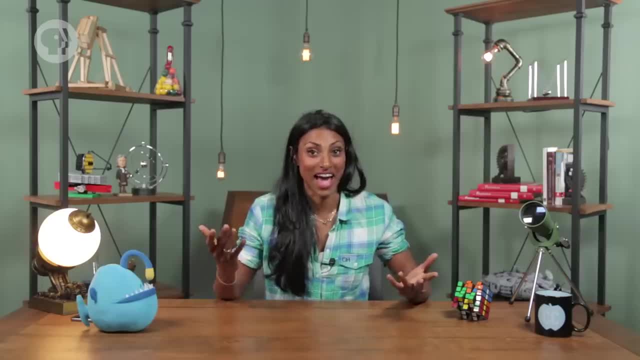 But of course, not all objects work that way. If you've ever tried to fling a hammer, for example- which I don't recommend doing- it wouldn't fly through the air in the same way a softball would, because the hammer's 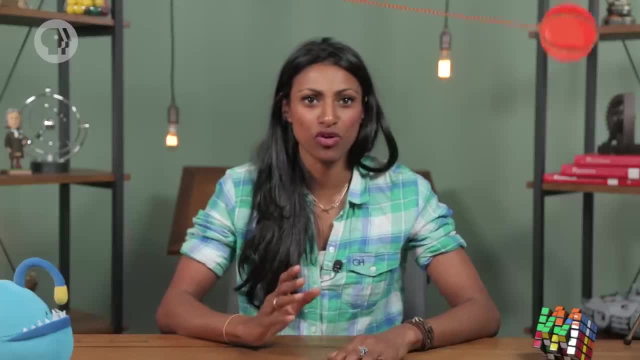 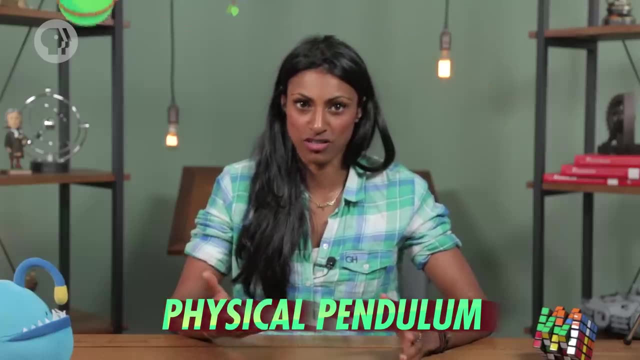 mass isn't distributed evenly. Likewise, a pendulum with a big ball on the end of a very light string called a simple pendulum, would behave very differently from a pendulum that uses a heavier stick, what's known as a physical pendulum. 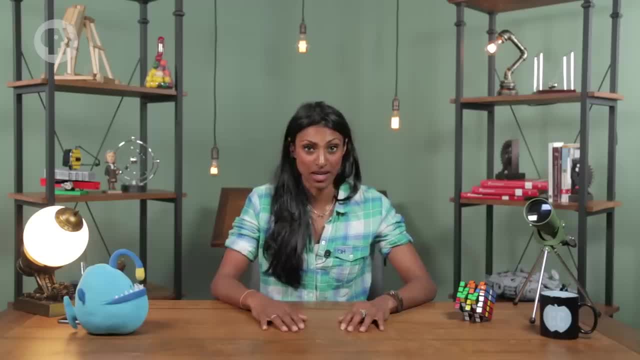 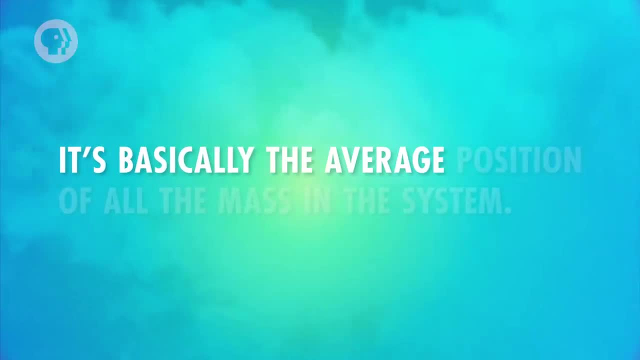 In these situations, it's more useful to describe what the center of mass is doing. When you throw a hammer, for example, it's going to rotate around its center of mass. So what is center of mass? It's basically the average position of all the mass in the system. 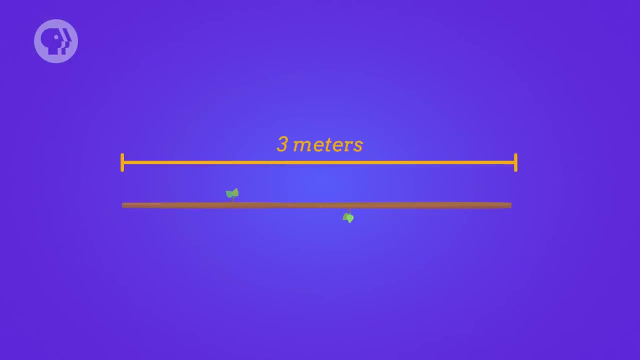 Say, you have a 3-meter-long stick, which we'll pretend is massless, with a 2-kilogram ball stuck on either end. It's easy to see where the center of mass should be. The mass is distributed symmetrically, so its center is going to be right in the middle. 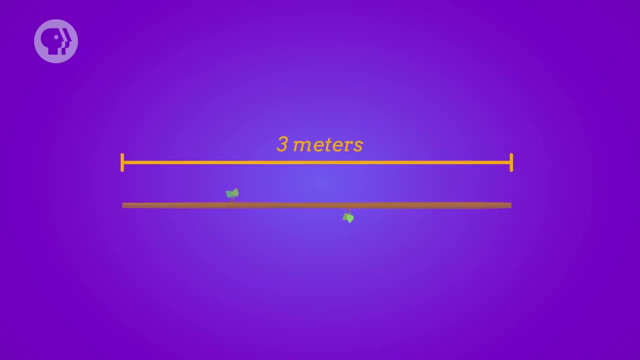 of the stick. Now let's say you have another 3-meter stick and on the left side there's a 2-kilogram ball and on the right side there's a 4-kilogram ball. So what is center of mass? 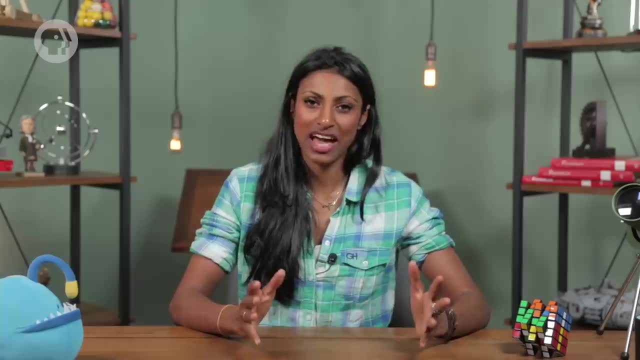 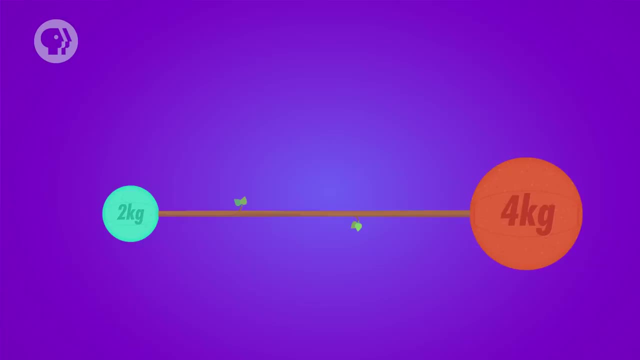 This time there's twice the mass on the right side of the stick. So when you're trying to calculate the average position of all the mass attached to the stick, you're going to be counting the right-hand side twice as much. That means the center of mass will be two-thirds of the way along the stick closer to the 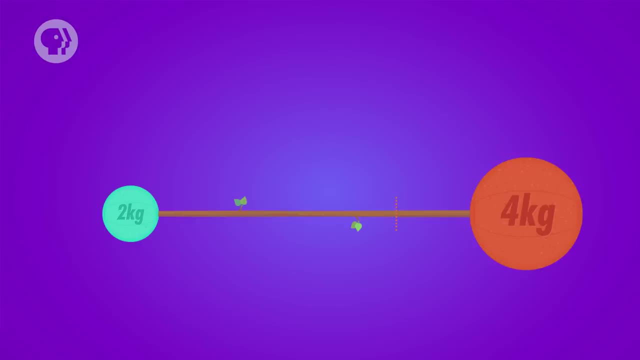 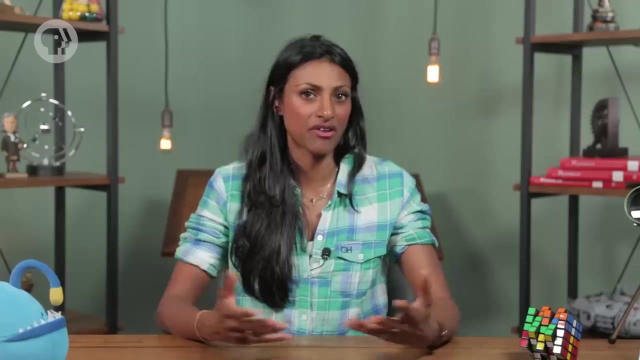 4-kilogram ball. It's like each piece of mass pulls on the center of mass a little bit, so parts with more mass end up pulling harder and moving it closer. But if you don't want to calculate this in your head, and if there are like seven,